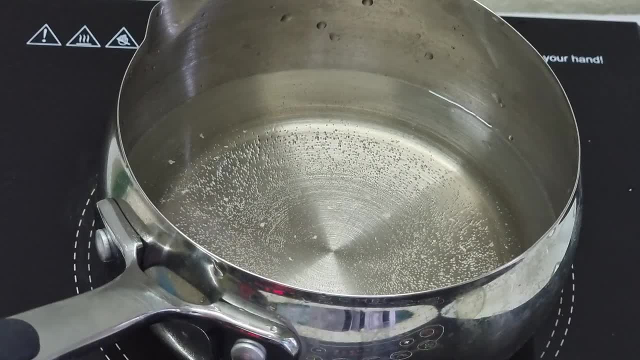 So as it reaches that point, then the water will start to evaporate. So as it reaches that point, then the water will start to evaporate. So as it reaches that point, then the water will start to evaporate. 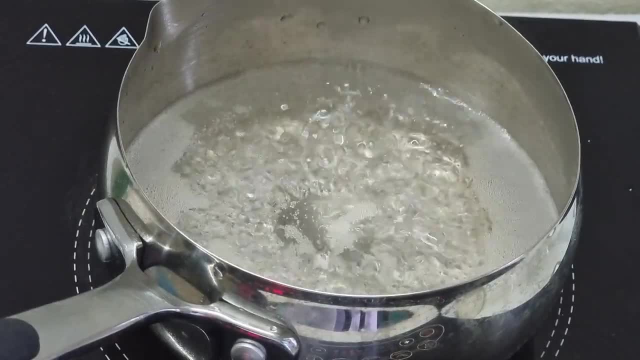 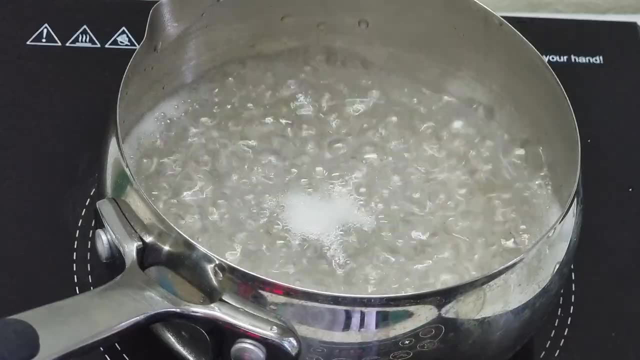 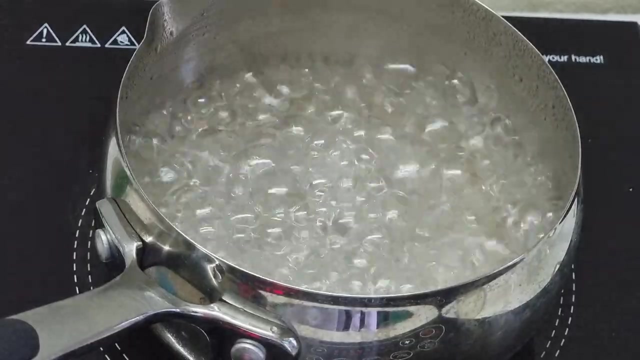 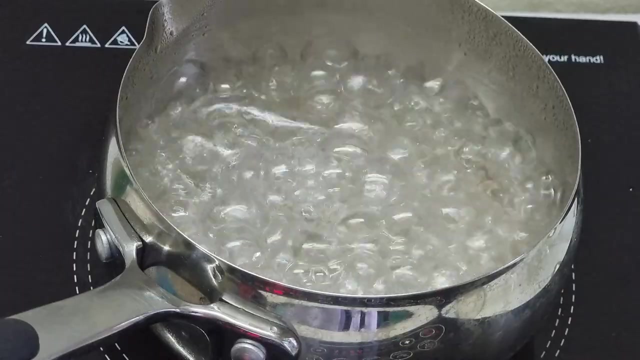 From our mixture. Okay now, so our solution is starting to boil. I think I used a lot of water for this, So it will take a while before all the water will evaporate from the mixture. So let's just wait. 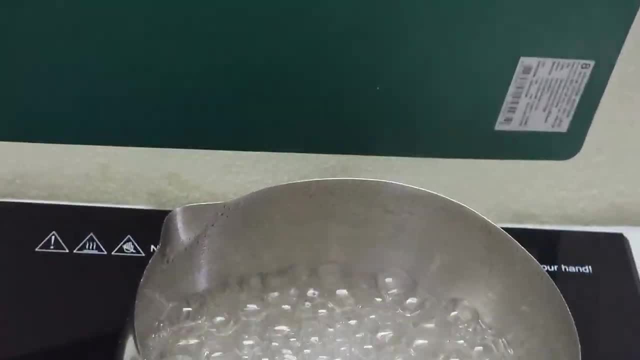 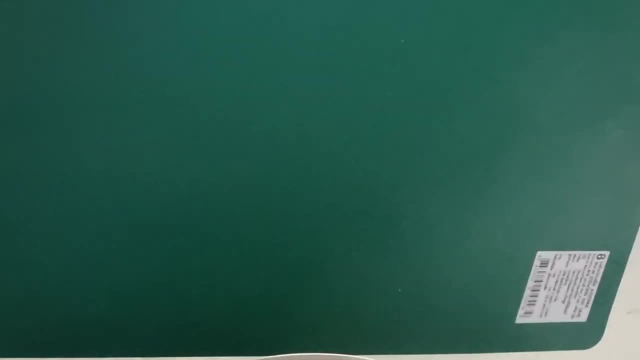 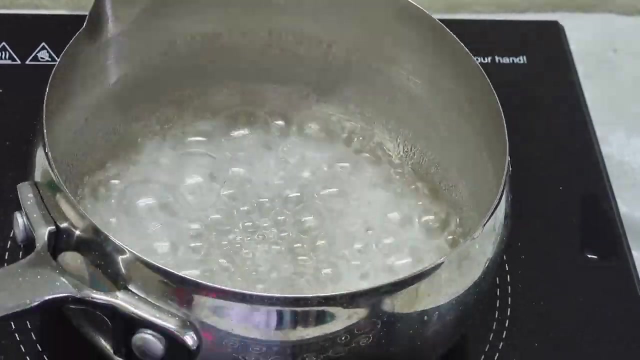 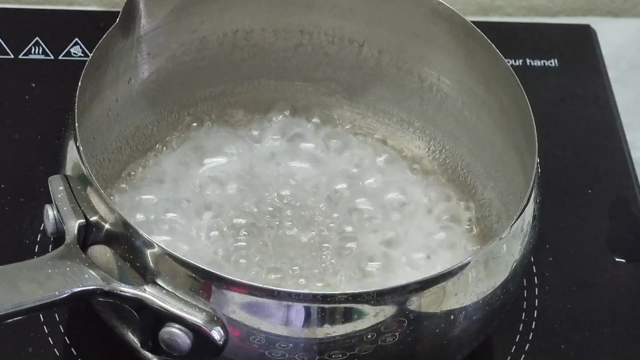 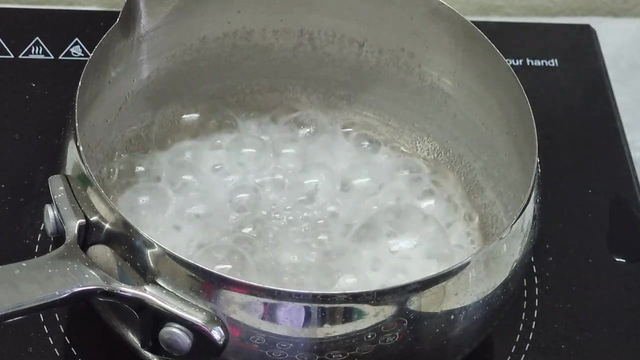 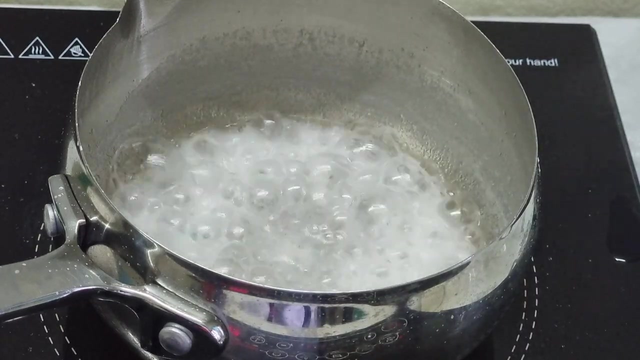 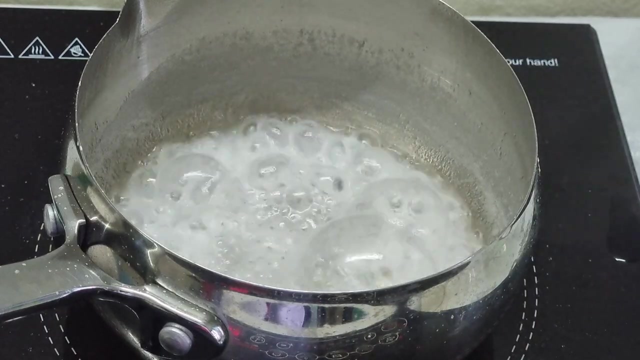 Okay, so you see all this vapor. okay, that's the water evaporating. okay, so you see all the water, all of the water. almost all of it has evaporated already and I think we can see. I think that's the salt. okay, the white one. so let us wait a little more. 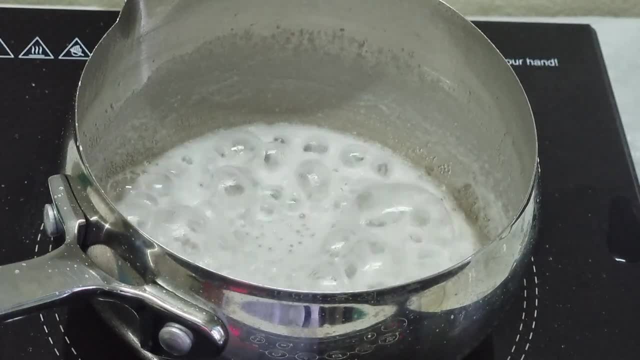 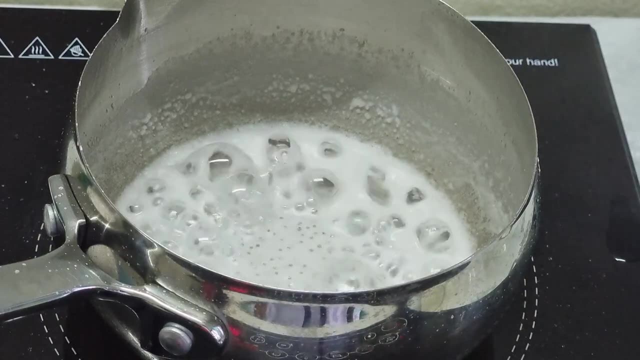 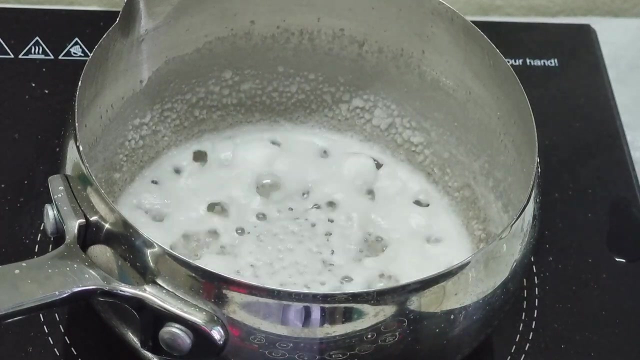 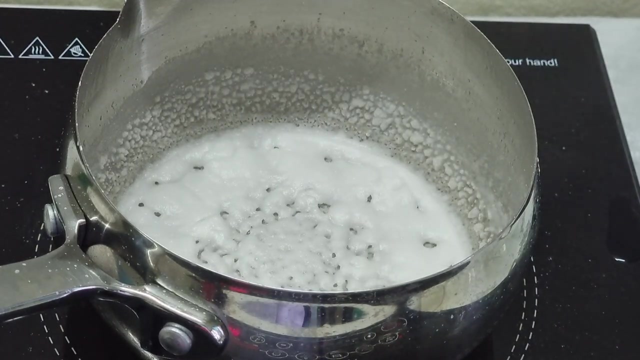 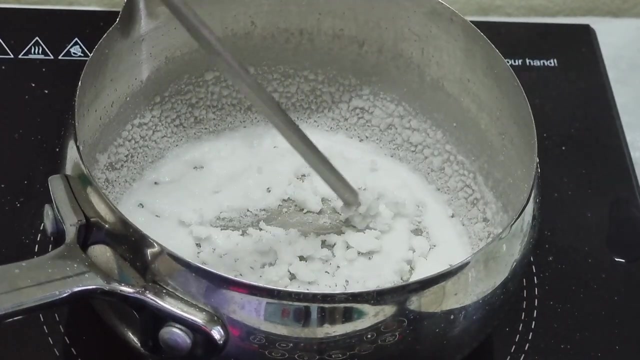 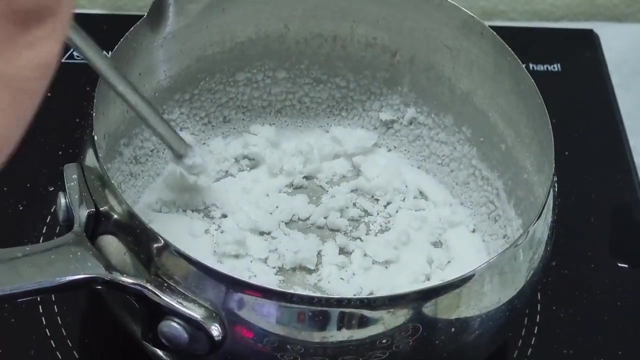 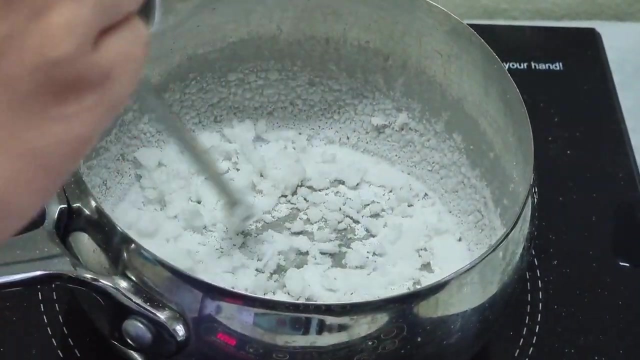 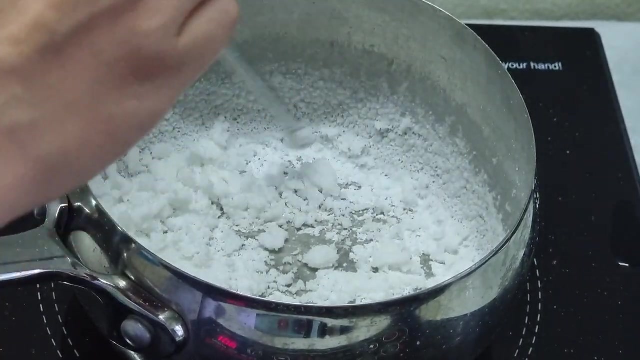 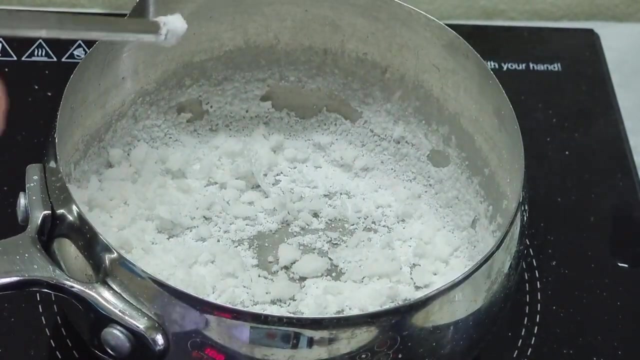 Okay, then the water evaporates and what will be left in our solution is the salt. okay, so that's how you separate salt and water, you see? Okay, so the water evaporated already and what's left behind? what's left behind is our salt. okay, so it's all dry, it's all dried up. okay, I think it's all dried up, okay, so let us wait a little more.